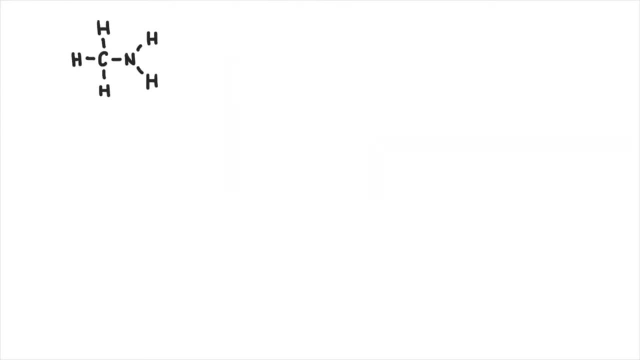 So let's do some naming. Identify the longest carbon chain. in this case it's methane. drop the letter E and replace it with amine. The amine functional group is given priority, so any alkyl groups are named according to standard conventions from this position. 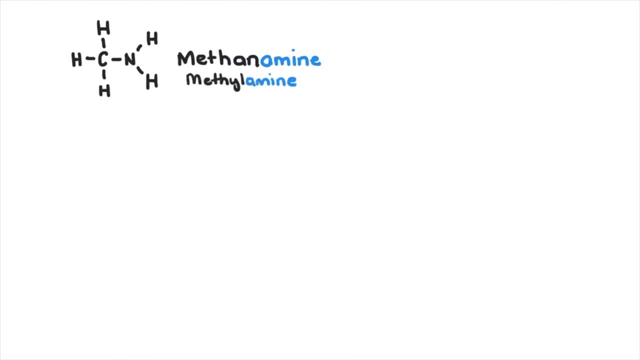 So this amine will just be called methanamine. Methyl amine is also acceptable, as it really is just a methyl group attached to the functional group. Let's grow this chain. The longest chain in this example contains three carbons, so we know its parent chain is propane. 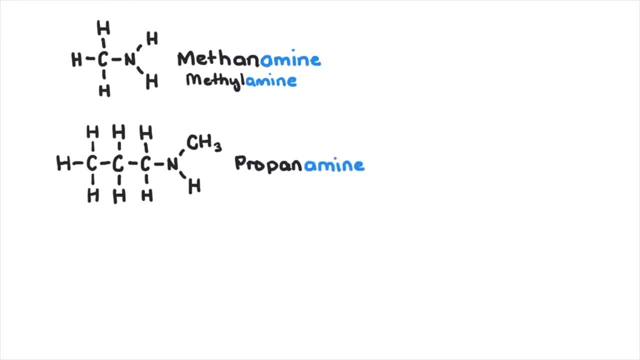 Drop the E and change it to amine. There's also a methyl group attached to the functional group And since these substituents are numbered from the functional group, there's no need to identify the position, as it's always at the start anyways. 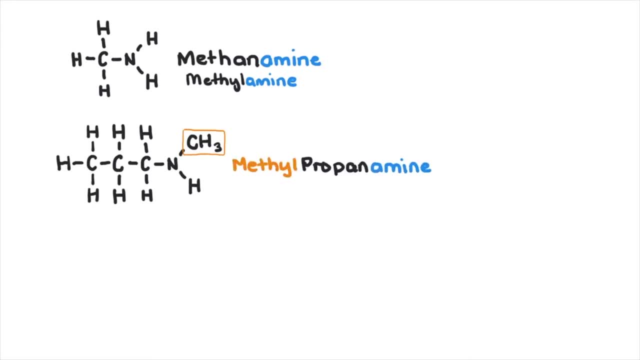 So this becomes methyl propanamine. Okay, next level, The longest chain, is butane. drop the E and replace it with amine. It also contains a methyl group here and here, Since the amine is given priority, we'll number the carbons, giving it the lowest possible position. 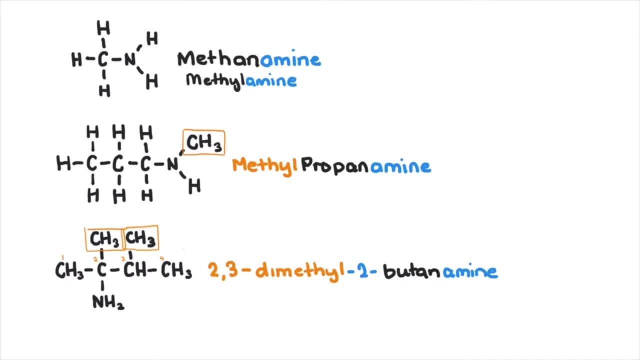 So this becomes 2,3-dimethyl-2-butanamine. Okay, last one. Well, it looks like there are three methyl groups attached to the nitrogen. This is called trimethylamine. There's no real parent chain here. 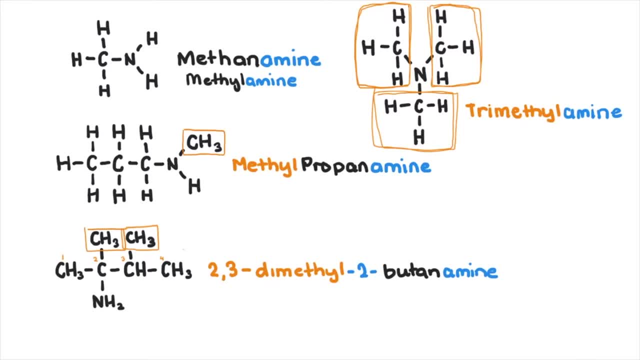 Amines can be further classified as primary, secondary or tertiary, just like the alcohols. These are known as primary amines as they only have one alkyl group attached to the nitrogen. This one is a secondary amine as it has two alkyl groups. 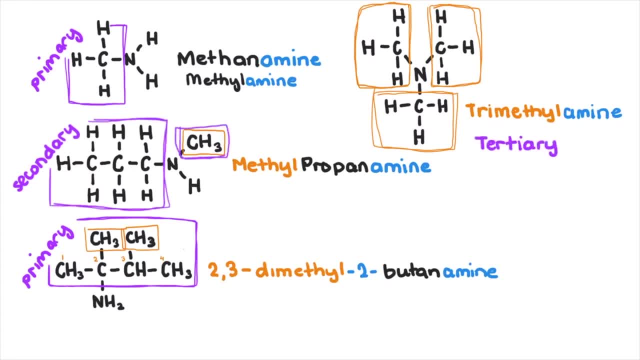 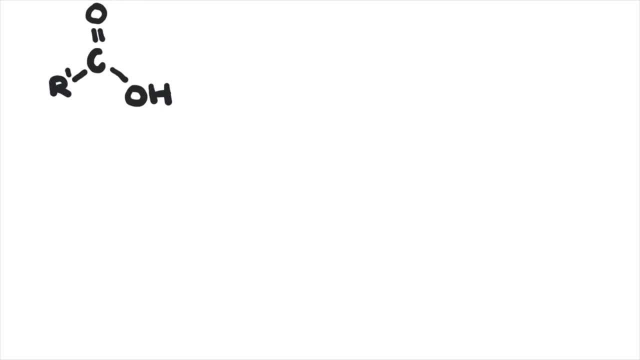 So what about the amides? If you take a carboxylic acid and replace the hydroxyl part with an amine, you get an amide. These have these general structural formulas where each R can either be an alkyl group or a hydrogen atom. 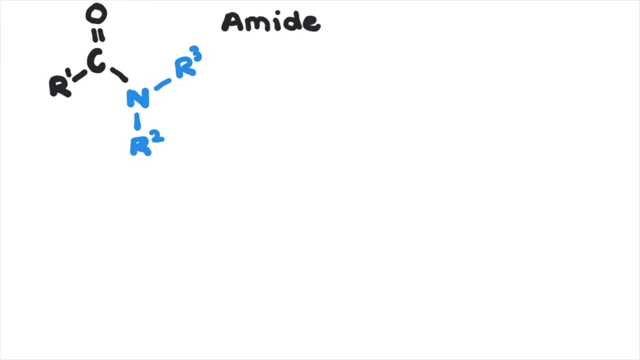 Have a geese at this one. The longest chain that contains the amide functional group is ethane, So drop the E and replace it with amide, So this becomes 2,3-dimethylamine. This is called tertiary amine as it has three alkyl groups attached to the nitrogen.